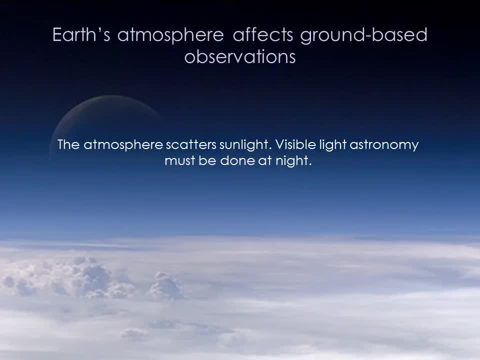 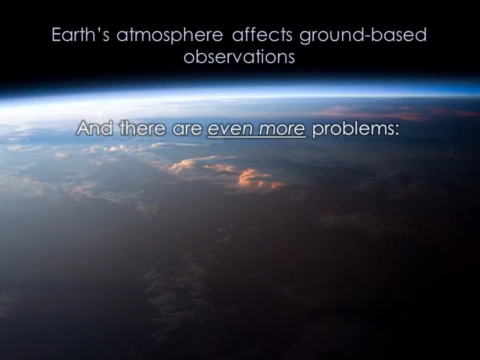 The much dimmer light of most celestial objects gets drowned out. so visible light astronomers can only work at night, And they can only work if it's clear. The sky is often filled with those pesky clouds. But even if it's at night and spectacularly clear, there are additional effects that stymie the astronomer. 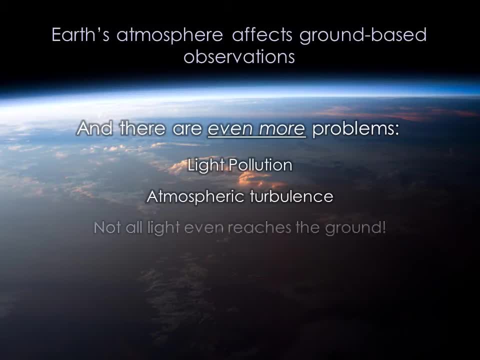 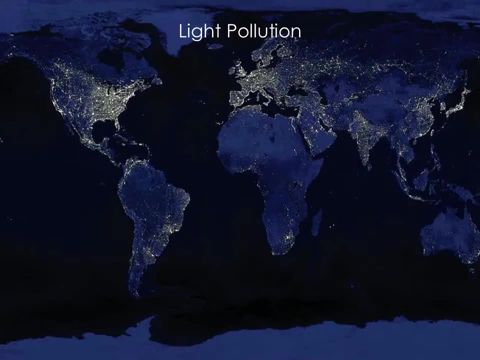 Light pollution, atmospheric turbulence and the fact that most forms of light can't even reach the sun. Just as our atmosphere scatters sunlight in the daytime, it also scatters city lights at night. We call this light pollution. Human-produced light pollution hinders our view of the stars and negatively affects astronomical research. 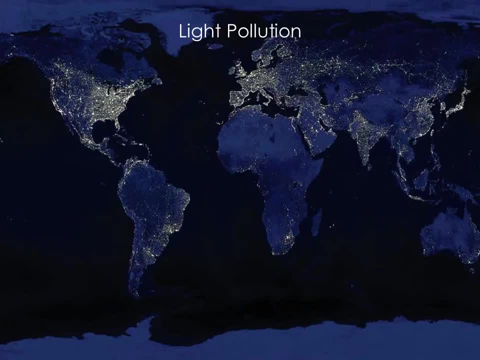 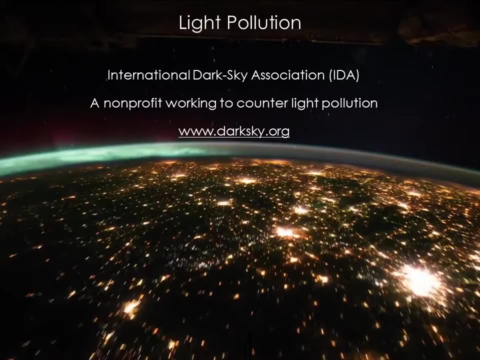 But it's also an environmental problem. Light pollution disrupts ecosystems, it affects human circadian rhythms and it wastes energy. It's estimated that approximately 50% of the Earth's atmosphere is light. Unfortunately, 2.2 billion dollars per year is lost due to poor lighting in the United States alone. 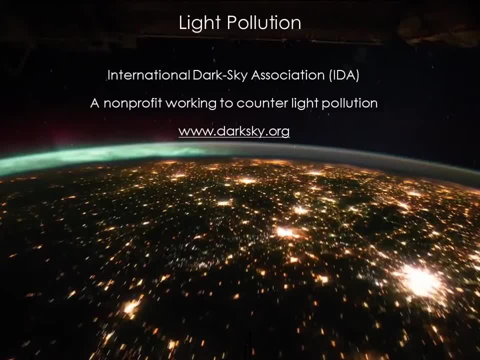 And the problem of light pollution is only getting worse. If you're interested in the issue of light pollution and how to fix it, the International Dark Sky Association is a non-profit that works to counter light pollution. Information on the IDA can be found online at darkskyorg. To understand turbulence. imagine a penny at the bottom of a very still pool. It's easy to see. Now imagine someone does a cannonball into the pool. The water gets wavy and the image of the penny jumps around. Being on Earth under the atmosphere is sort of like being at the bottom of a pool. 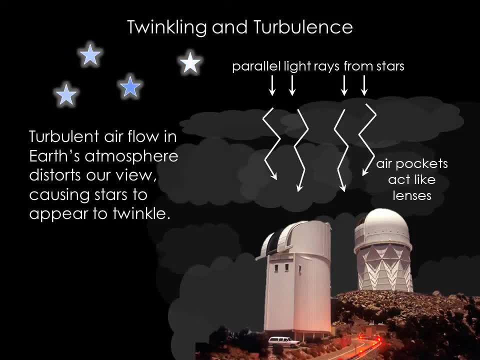 To do astronomy we have to look through layers of air. The more still the air is, the easier it is to see the stars. The uneven heating and cooling of the atmosphere creates moving bundles or pockets of air. These air pockets act like little lenses. 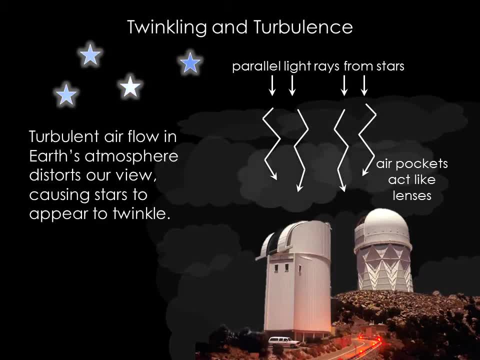 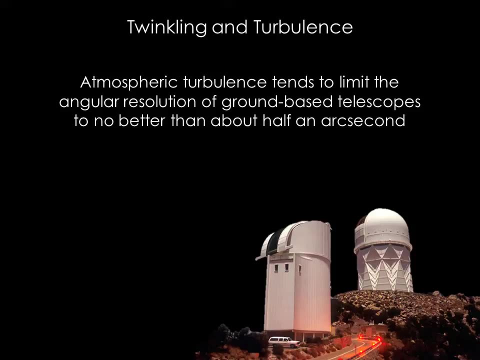 When parallel light rays from a star hit the bundles, the rays bend in unpredictable ways. Therefore, when a telescope on the ground looks up at the night sky through the atmosphere, we get a twinkling and blurry image. Atmospheric turbulence tends to limit the angular resolution of ground-based telescopes. 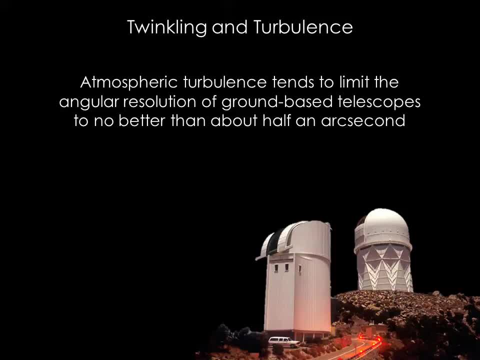 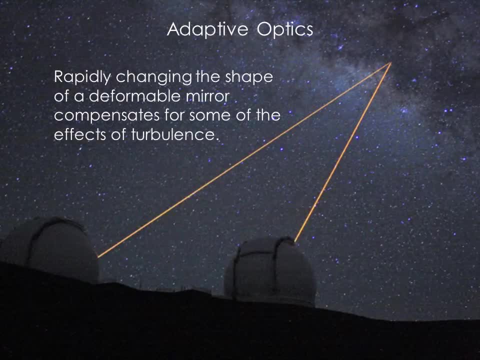 to no better than about half an arc. second, even if a telescope theoretically can achieve a smaller angular resolution, One technique to counter turbulence is called adaptive optics. Sophisticated deformable mirrors controlled by computers can correct in real time for the distortion caused by the turbulence of the Earth's atmosphere. 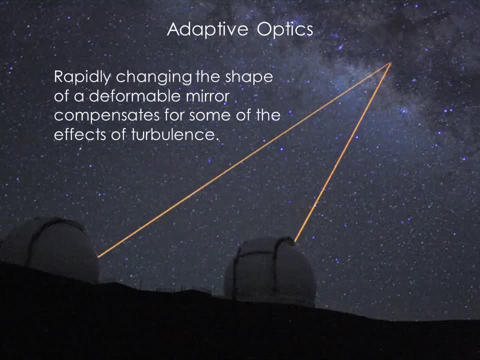 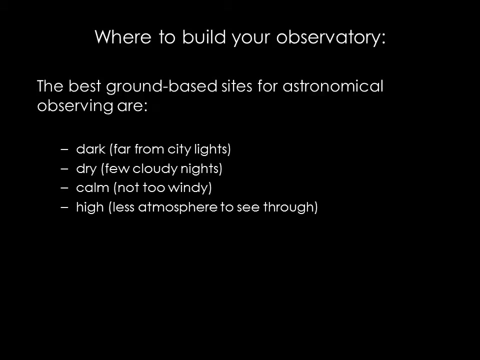 A computer calculates the necessary changes by monitoring distortions in the image of a bright star near the object of interest. If there is no bright star nearby, a laser is used to create an artificial star to monitor the distortions When you're choosing the location of the next great Earth-based observatory. 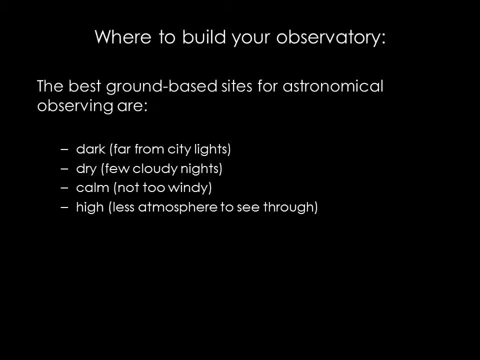 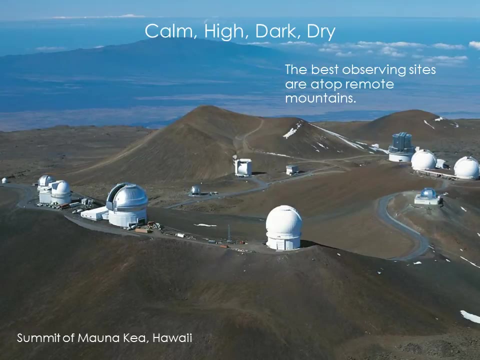 you want to minimize the effects of bad weather, light pollution and turbulence as much as possible. The best sites are dark, dry, calm and high above the densest parts of the atmosphere. There are some sites around the world that meet these criteria. 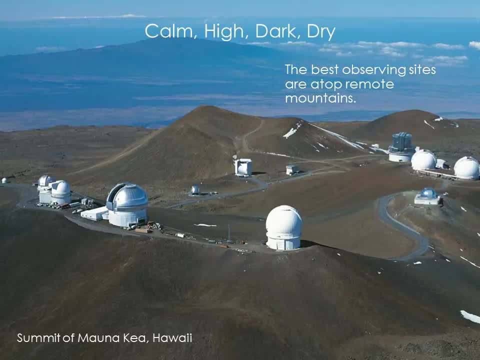 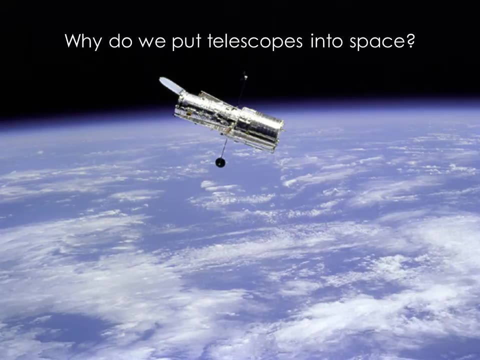 For example, the 4,300-meter summit of Mauna Kea in Hawaii. Of course, the best solution to our atmospheric troubles is to put our telescopes into space where there is no daylight, no clouds, no light pollution and no turbulence. 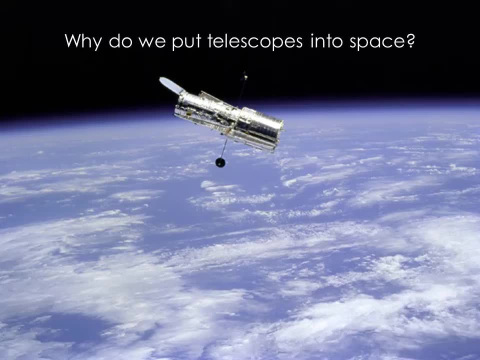 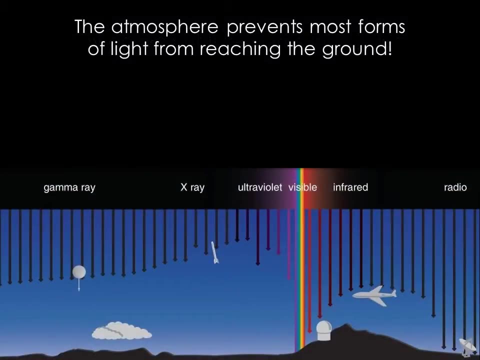 This is why the Hubble Space Telescope, despite its modest mirror size of only 2.4 meters, has been so enormously successful. But there's another good reason to put telescopes outside of Earth's atmosphere. Earth's atmosphere poses a problem that no ground-based telescope can overcome. 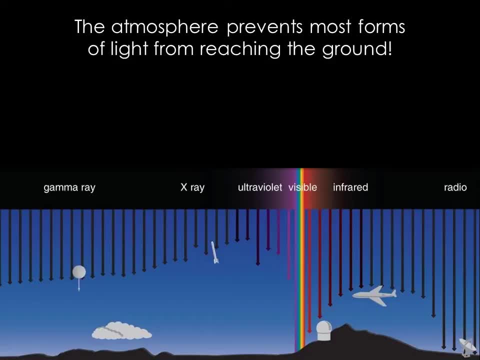 Our atmosphere blocks most forms of light. Astronomical phenomena emit light at all energies of the electromagnetic spectrum. so of course we want to look at everything, Only we can't, at least not from the ground. This figure shows the approximate depths to which different forms of light penetrate our atmosphere. 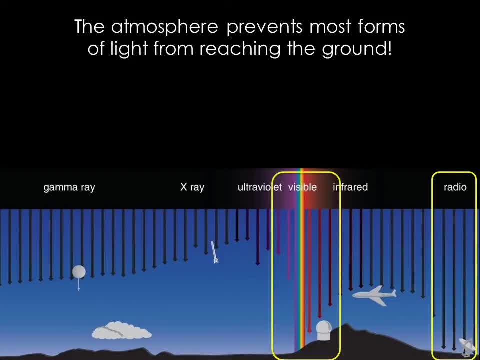 Only radio waves, visible light and the very longest wavelengths of ultraviolet light and small parts of the infrared spectrum can be observed from the ground. Therefore, the most important reason for putting telescopes into space is to allow us to observe the rest of the electromagnetic spectrum. 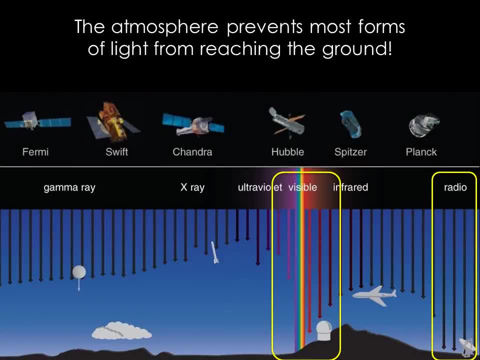 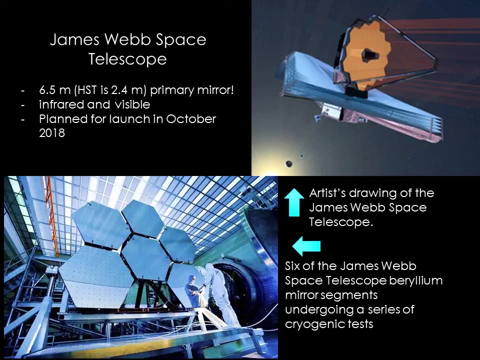 The Hubble Space Telescope is probably the most famous observatory, but there are many others that operate in parts of the electromagnetic spectrum that do not reach the ground. NASA plans to launch an even more powerful infrared observatory. The James Webb Space Telescope will be the successor to the Hubble Space Telescope.